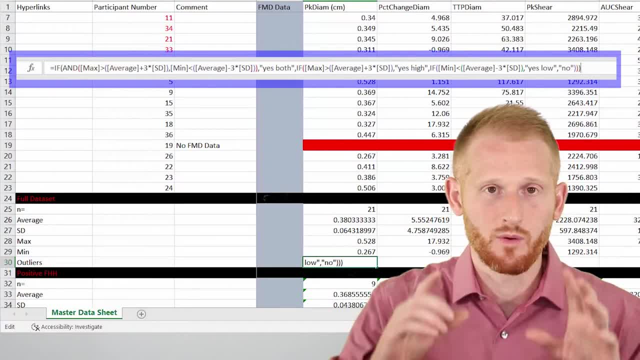 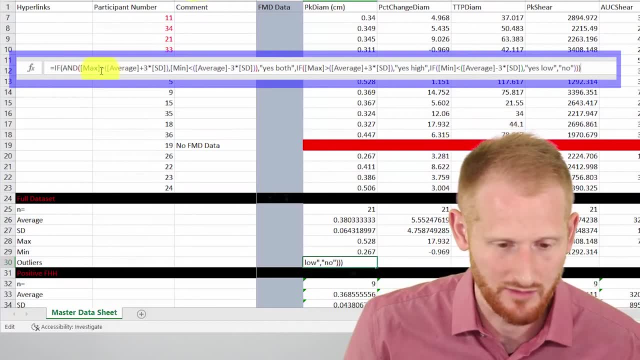 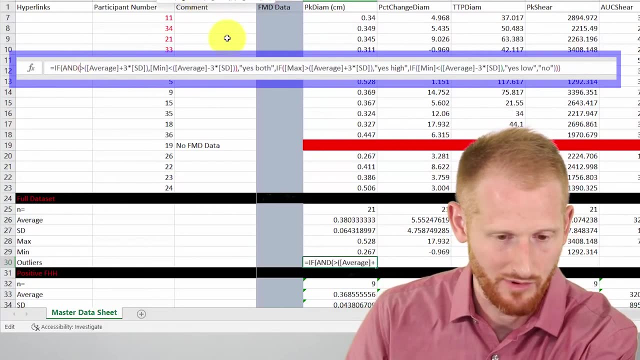 the variables that are within brackets, with whatever that whenever it says within the bracket. So, for instance, here we have within this set of brackets we have the word max. So we want to remove that. So get rid of the brackets and the word, and I'm going to click where the maximum. 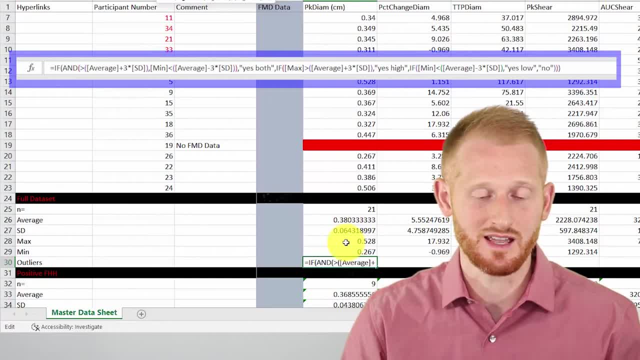 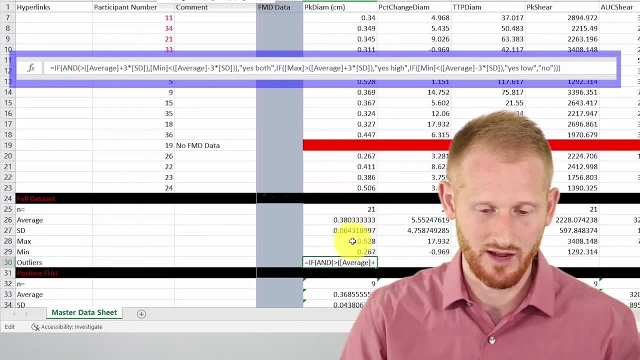 variable or the maximum value is, And then it hasintend that in that bracket. And then I'm is in this data set. so in the peak diameter the maximum variable or the maximum data was calculated right here, so 0.528. so I'm going to click that. 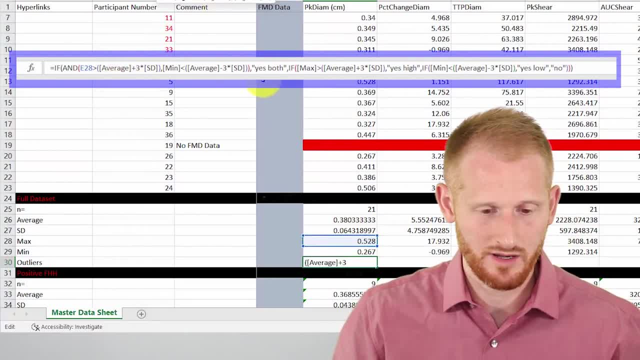 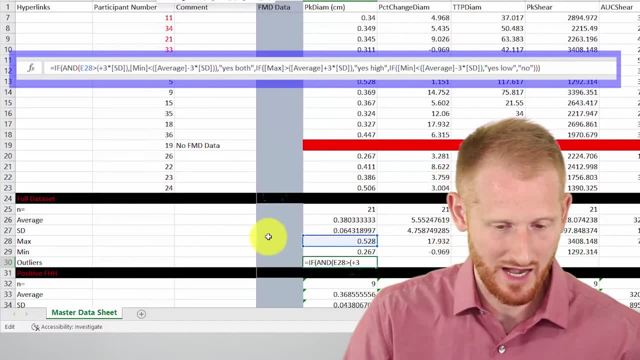 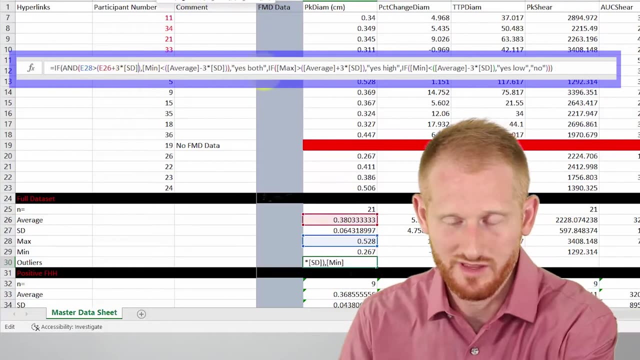 alright. so the next one is where it says average. so again, I'm going to get rid of the bracket and the word average in the opening bracket and I'm going to click where the average is. I'm going to do it again for the standard deviation. so what? 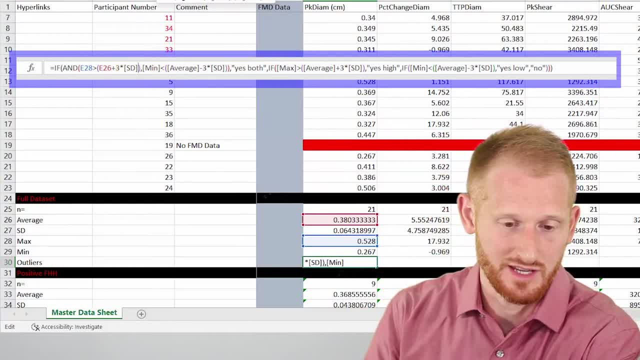 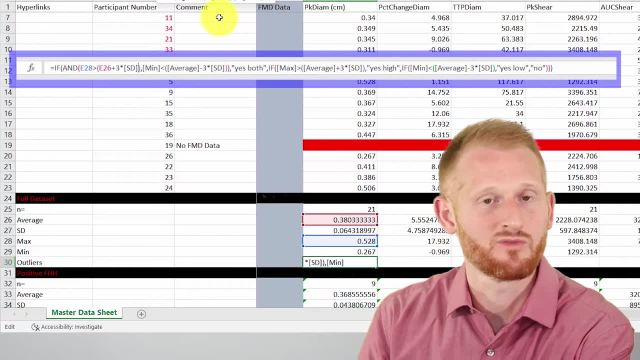 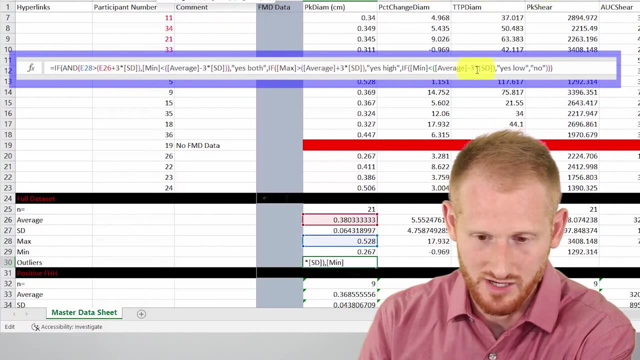 this is actually going to be doing is gonna. it's going to be calculating three standard deviations above and below the average and then it's going to look and see if your minimum and maximum values, or beyond that, you can change this number three here. you would also have to change it right here and change it right. 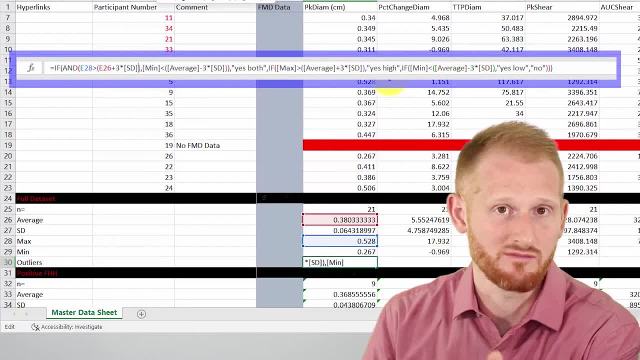 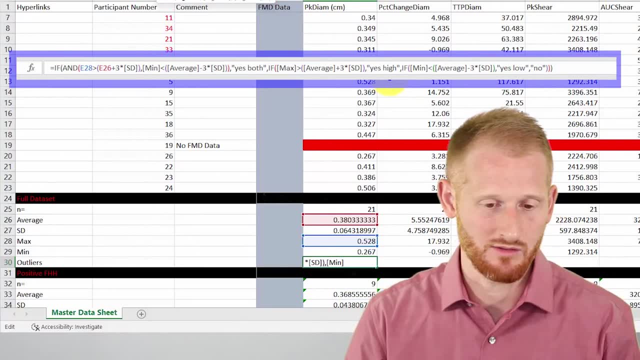 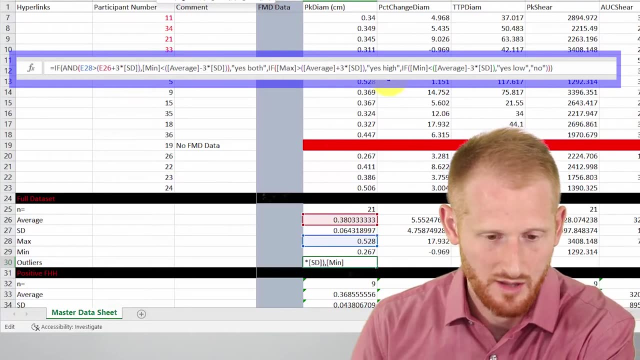 here to another number. so you can do two standard deviations. so you just change those threes into twos. you can do four standard deviations by changing the threes to fours. however you want to do that. um, three is fairly standard. a lot of people use three standard deviations, so but 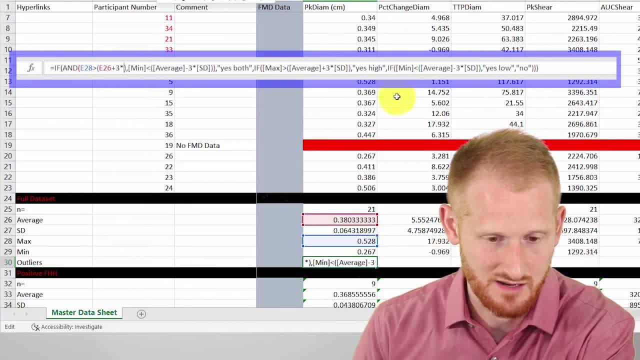 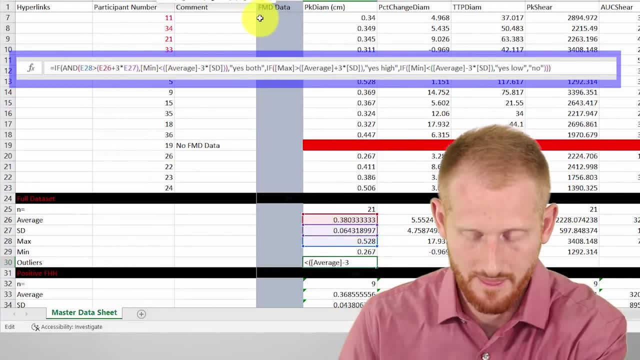 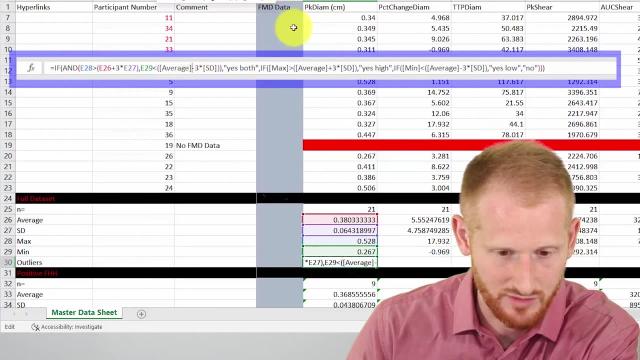 let's remove again the bracket, this SD, which stands for standard deviation, and we'll click right here where our standard deviation is. here's another, here's a minimum. so, again, let's get rid of that, click where the minimum is. and we're gonna be doing this a handful of times, alright, so this seems like a lot. 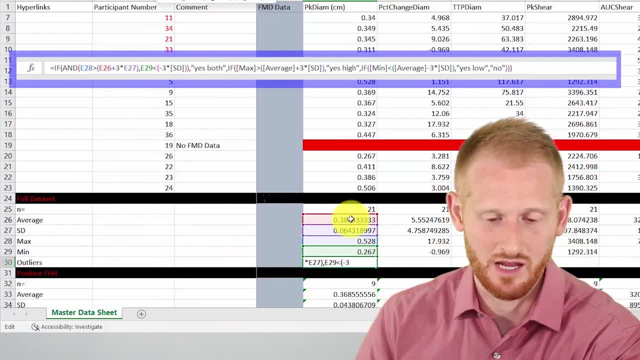 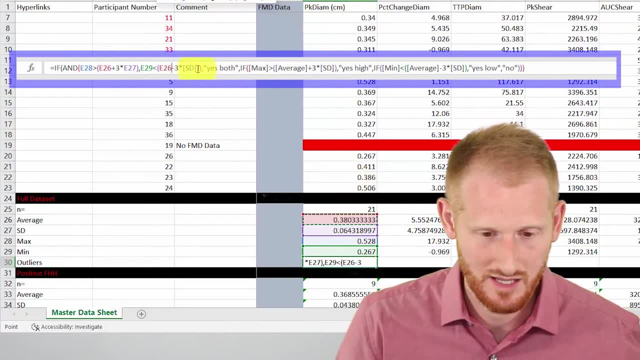 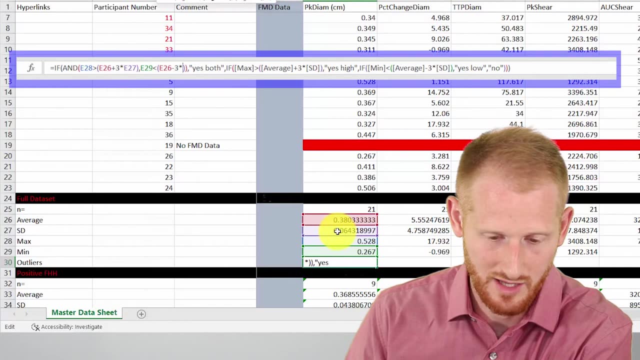 of work, but I promise you doing it this way is much easier than typing the entire formula in from scratch, which is what I had to do initially, when I sort of made this: let's get rid of the standard deviation, and with it the abbreviation for it, and put in the actual same deviation. here's a max get. 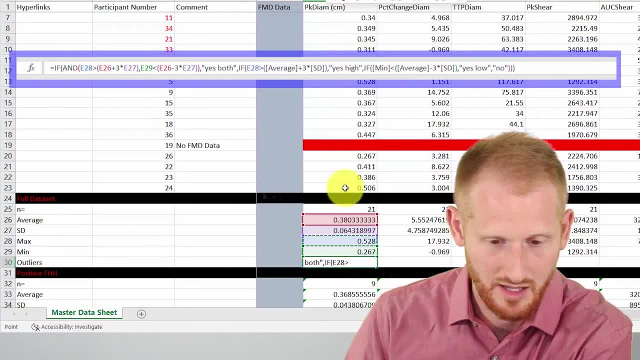 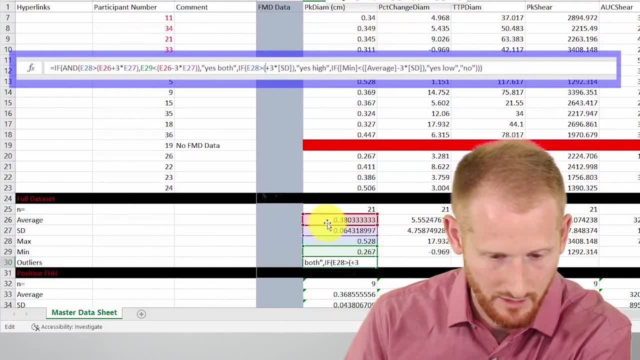 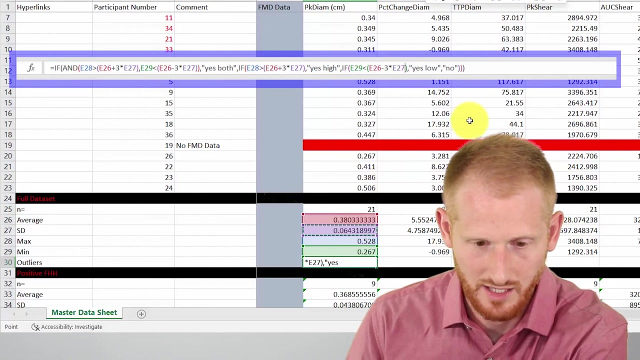 rid of. that's here's. our maximum value is right here, our average. rid of the bracket in the word is right here, And we have to do this several times. So standard deviation, minimum average here, standard deviation, and I think we got them all now So I can hit enter and it's. 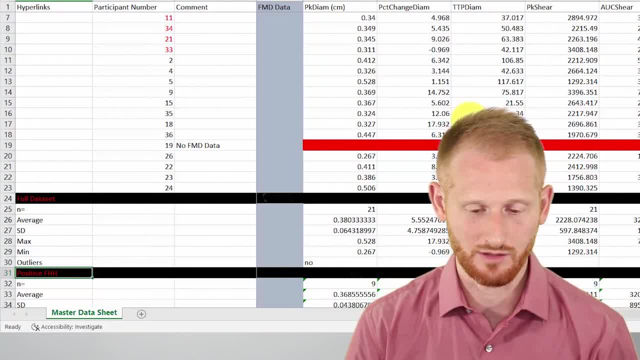 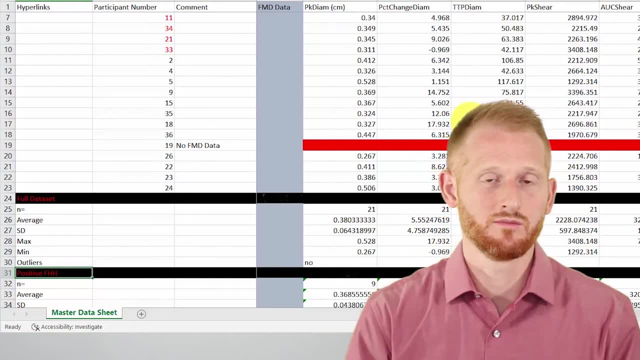 going to tell me. no, there are no outliers in this data set based on the averages, the standard deviations and how far away from the average the minimum and maximum value is. Again, it went three standard deviations above, so the average plus. 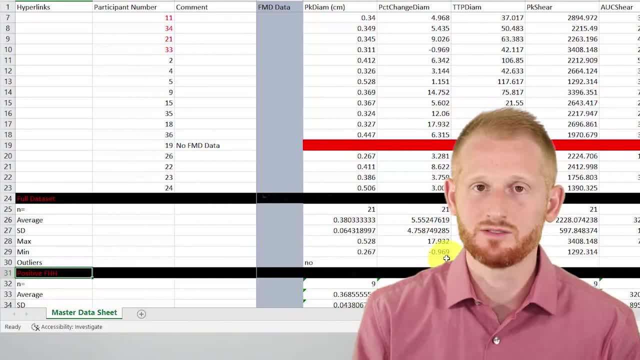 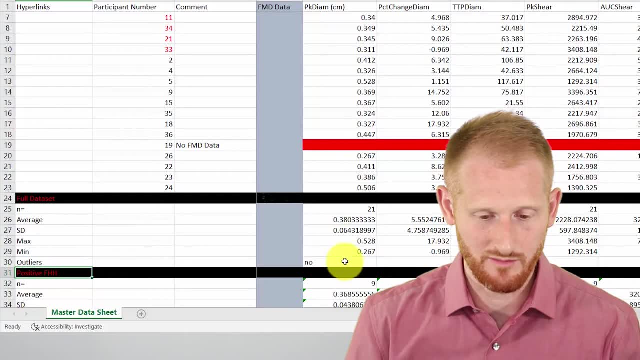 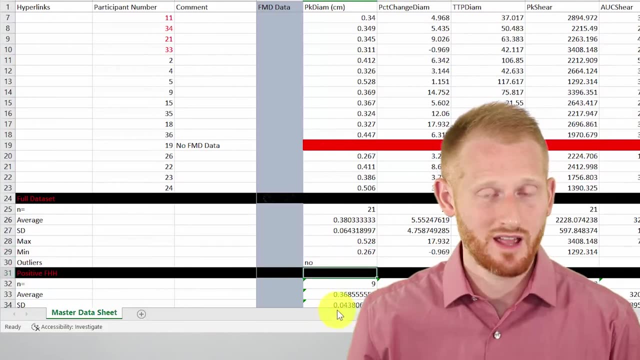 three standard deviations above. Was the maximum value above that? No, Okay, And also average minus three standard deviations below. Was the minimum value here below that? No, So we don't have an outlier above or below. So right now it doesn't say that there's. 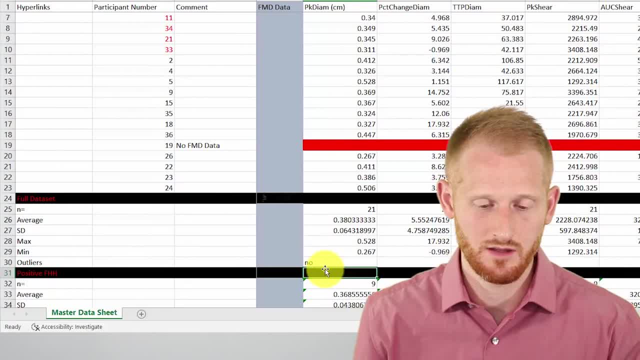 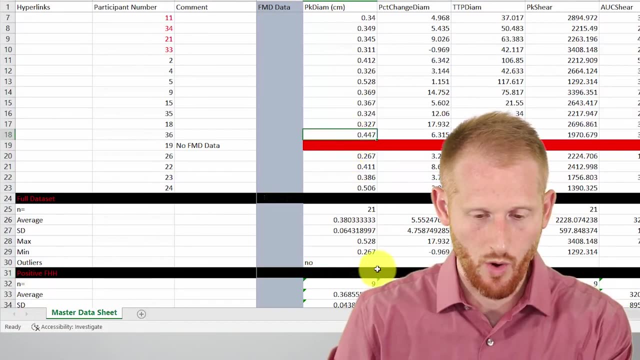 an outlier because there isn't one, statistically speaking, based on this justification at least. But let's force an outlier, just so you can see what that would look like. So the highest number here is 0.5.. 0.528.. Let's go up here and put a 100 in, All right? So I'm going to override this data. 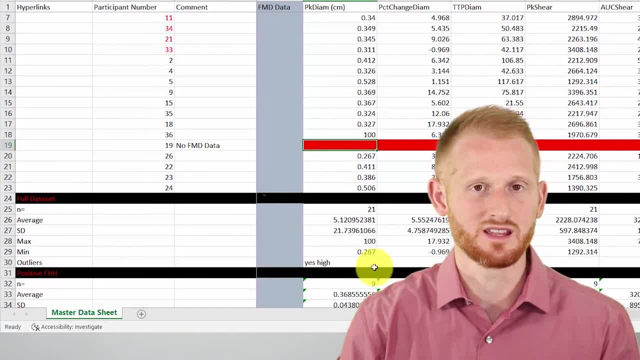 here And say I had a typo and I accidentally put 100 there instead of the 0.447 that was there. It's now going to warn me that there's an outlier. So it says yes, there's an outlier. 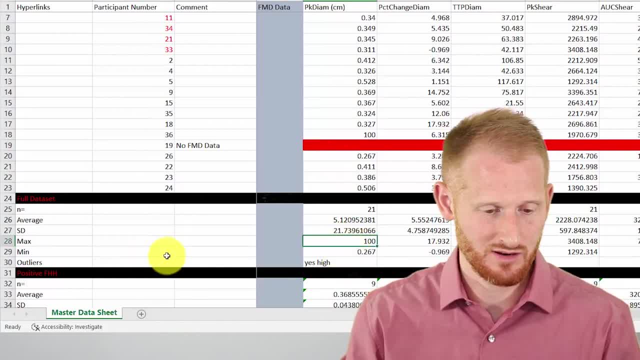 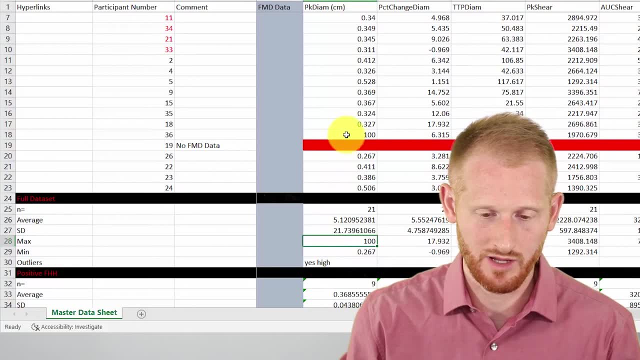 and it's high. Look at your maximum value here It's 100.. Hopefully you know a little bit about the data set and you know 100 is way too high. So you go and you look for that 100. And then you go and you look for that 100. And then you go and you look for that 100. 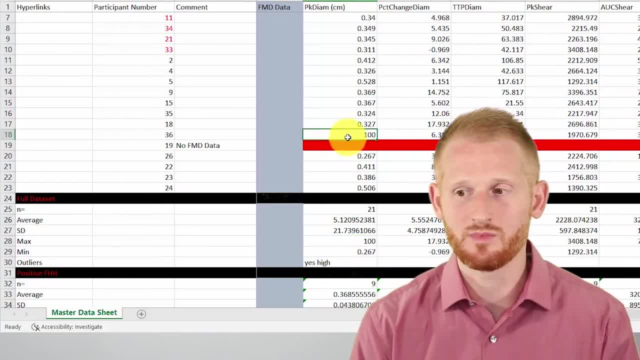 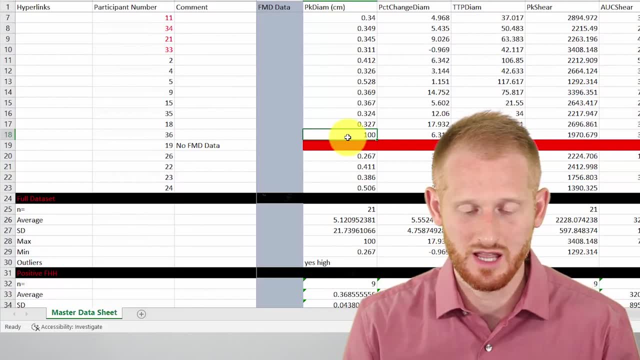 And then you go and investigate it and determine what's going on, whether it's a typo. maybe- hopefully- you have the data in some other place, somewhere so you can go back and find out if it's a typo of some sort and you can correct that. Let's say that there's also 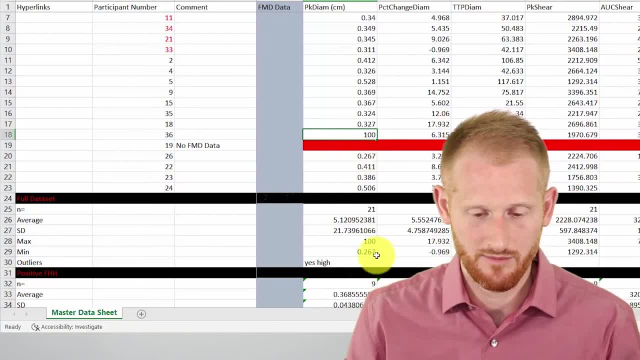 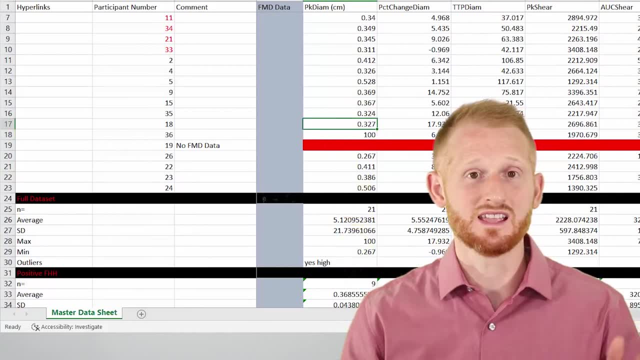 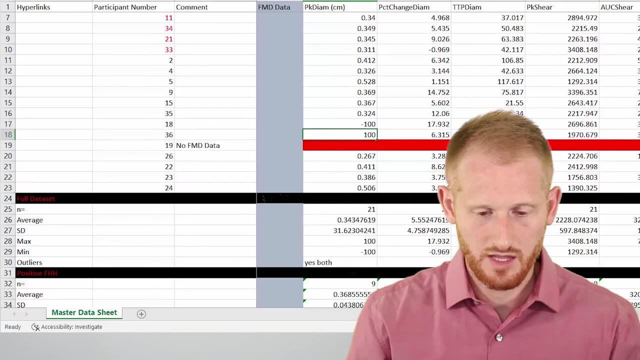 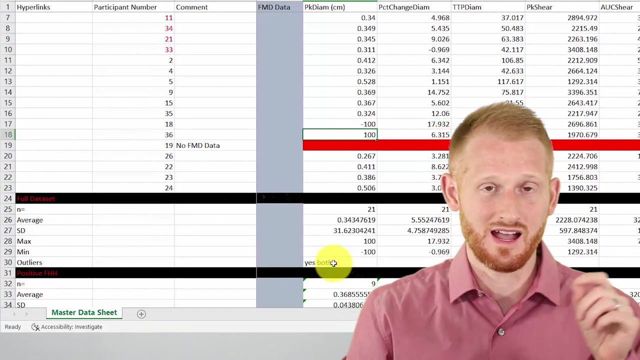 a low outlier. So the lowest value right now is 0.267.. Let's go to this one up here and let's put a negative value so we know it's going to give me an outlier. So we'll say negative 100.. Now it says yes, there's an outlier and it's both, Because we have a. 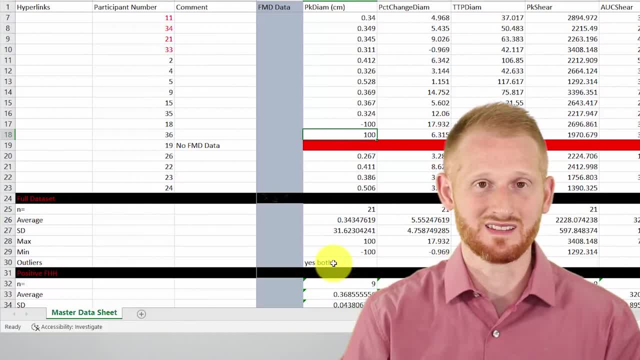 high outlier and a low outlier. we have two values at least, at least two values that are well outside of the expected values of within three standard deviations from the average. So you can see that the minimum is negative 100.. You know that there can't be. 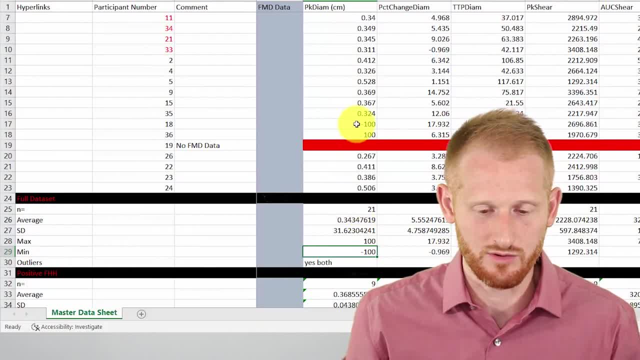 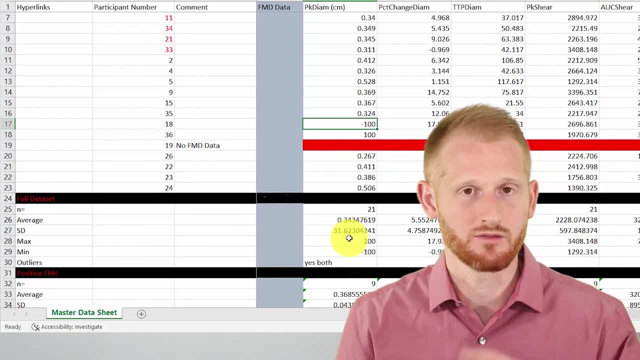 negative values in this variable, So you can see that the minimum is negative 100.. You go and you find that and then again you go and try to figure out why it's there. Hopefully it was a typo and you can correct it with the original data set. So let's get rid of. 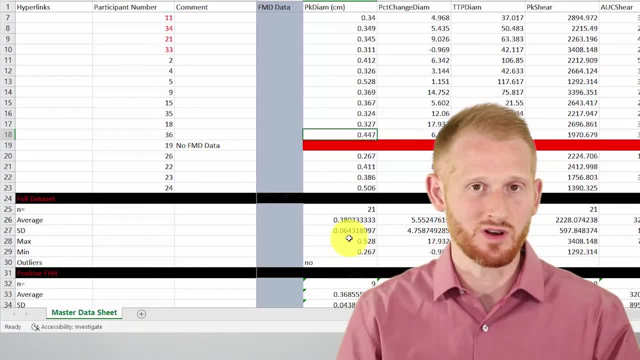 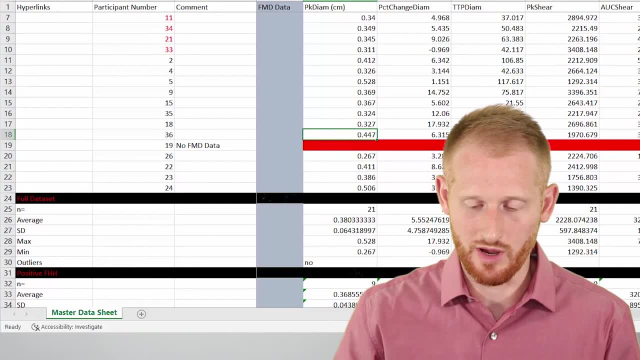 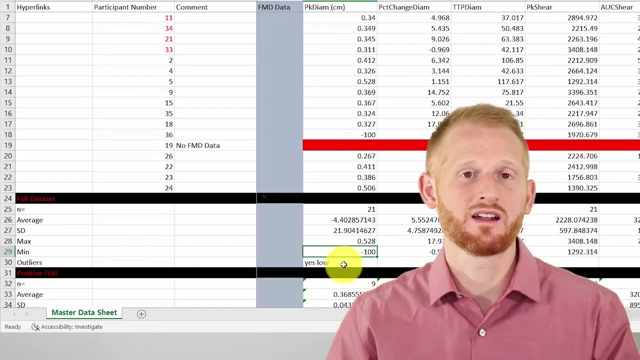 both of those. I just hit Control-Z twice to undo both of those fake numbers that it's put in there, Just so you can see if it is just a low outlier, let's do that one more time. So negative 100. It says yes, low, telling me there is an outlier and it's a. 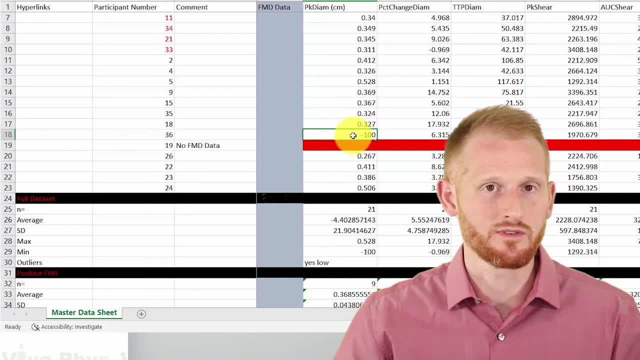 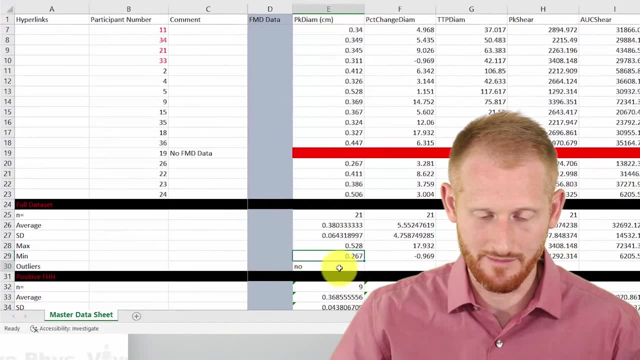 low outlier. So go look at your notes And then you can see that there's a low outlier minimum. Find that and go figure out why it's there. So I'm going to hit Control-Z again to undo that, because I don't want that in my data set. So let's copy this across and: 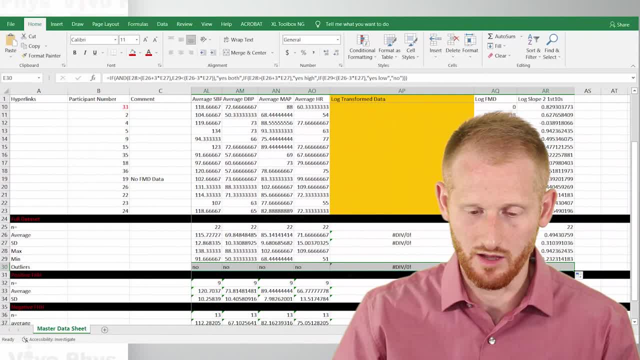 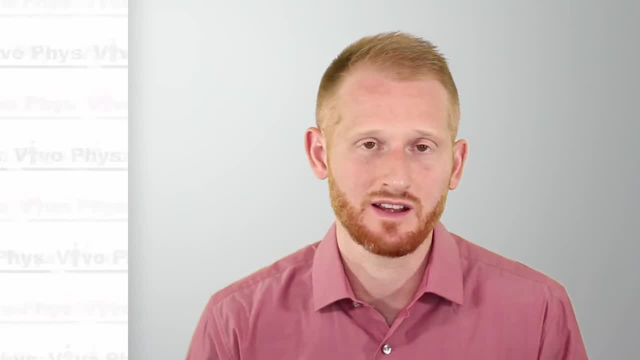 it will then do that automatically for every column of data we have. So you can see how you can very easily look for outliers. It's not a perfect system. It's not going to find every outlier in what is and is not an outlier. It has some subjectivity to it. It's going. 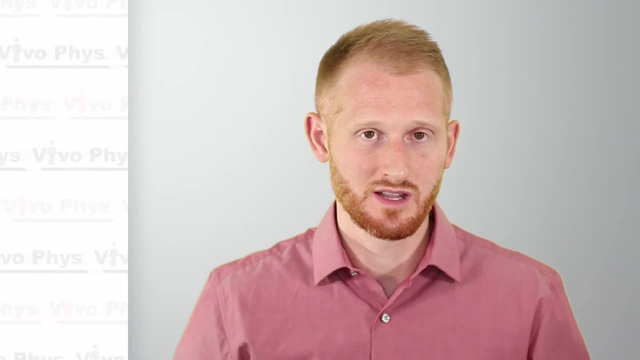 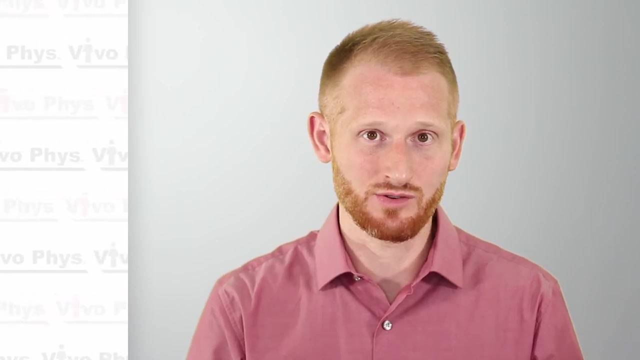 to find it. But this gives you an objective, upfront decision you can make for identifying potential outliers that you should at least go and investigate to see if it's an accurate number or if there was some sort of error that was put into the spreadsheet that you. 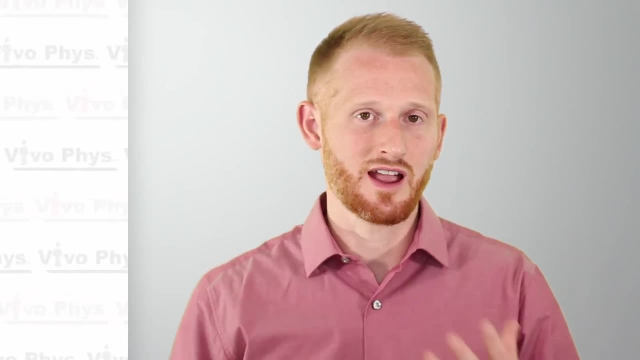 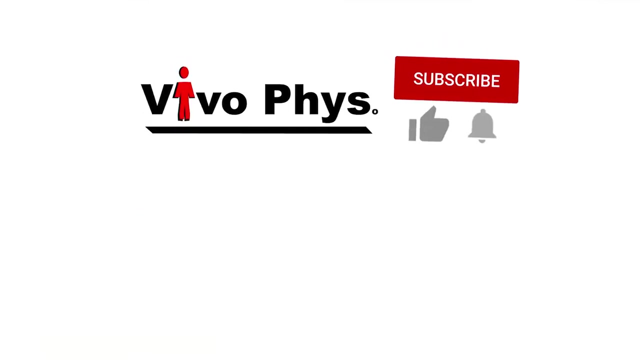 should correct. So now that you're pretty sure you have a clean data set, you can start actually doing some comparisons between the groups, So in this case between those with and without a family history of hypertension. So on the next video I'll be showing you how to do. 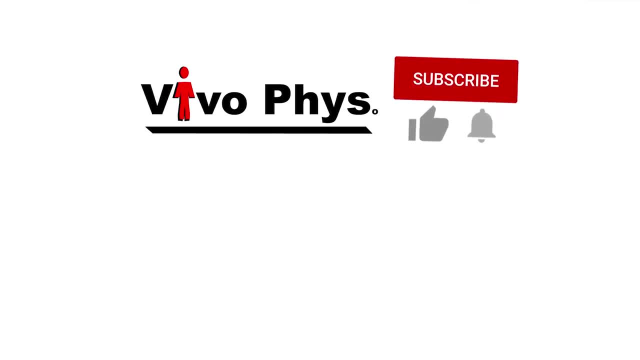 a very simple comparison Using a t-test function within Excel.